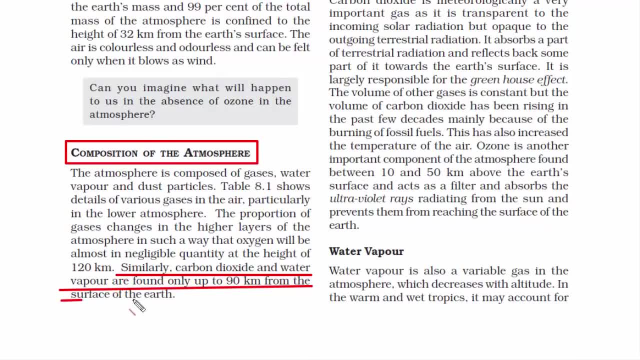 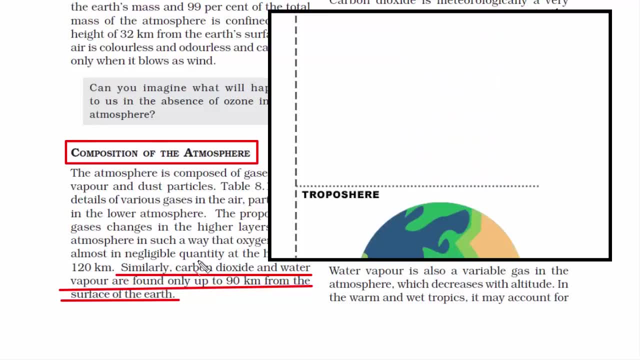 dioxide and water vapor are found only up to 90 kilometer from the surface of the earth. Let me just pull up the five different layers of the atmosphere. Here's the pick and you can see. the first layer, which is closest to the earth's surface, is troposphere, which exists up to 10. 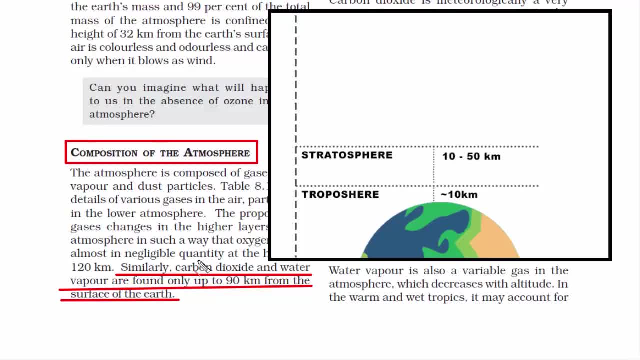 kilometer from the surface of the earth. After that we have stratosphere, then mesosphere, after that thermosphere and finally exosphere. So here when it says carbon dioxide and water vapor are found only up to 90 kilometer from the surface of the earth. 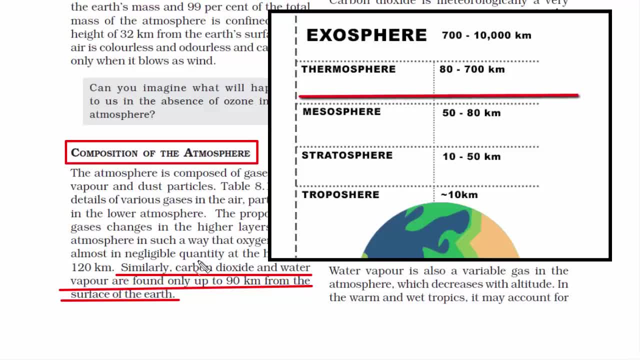 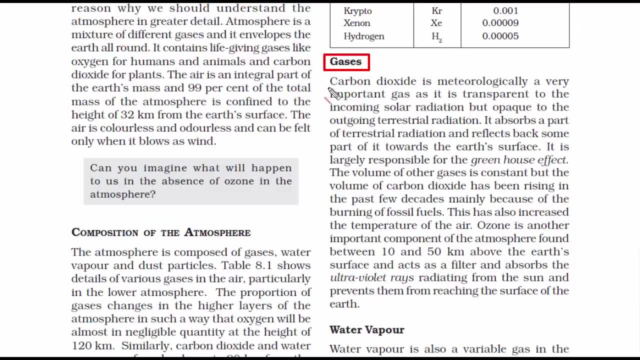 it means that carbon dioxide and water vapor exist till the initial boundary of thermosphere. I hope this part is clear now. Now let's read about this topic: gases: Carbon dioxide is an important gas. Remember this point. I'll get back to this. It is transparent for the incoming. 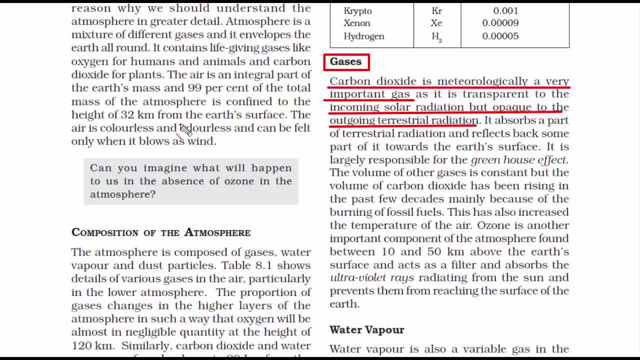 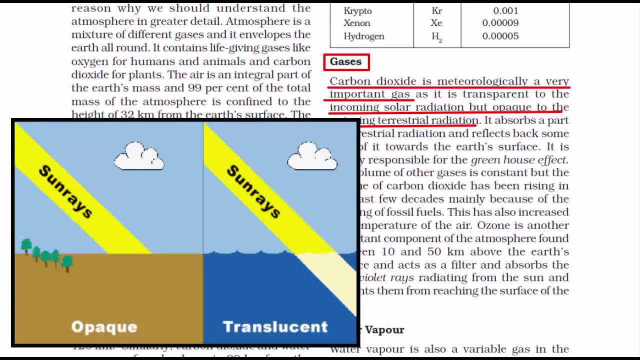 sun rays, but it is opaque to the outgoing terrestrial radiation. All right, let me just explain this line, what I just said. Now you must be aware of this phenomena, that differential heating of land and water is the reason behind rainfall and precipitation. Now, having said that, we now clearly know that earth's surface just gets heated up due to sun. 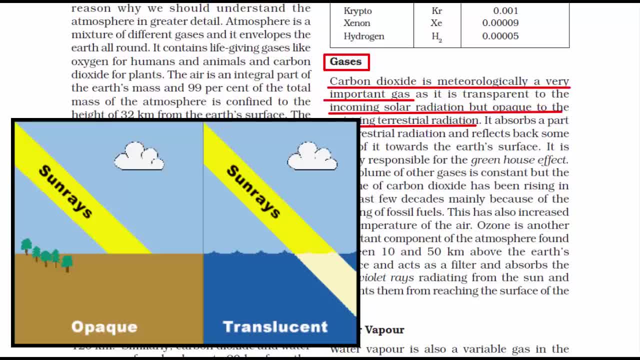 rays and because earth's surface heats up due to the incoming sun rays and that heat has to go somewhere. it is because of carbon dioxide. the heat is trapped within the earth's atmosphere. This is what is causing climate change. Now you must have heard about greenhouse gases. They are 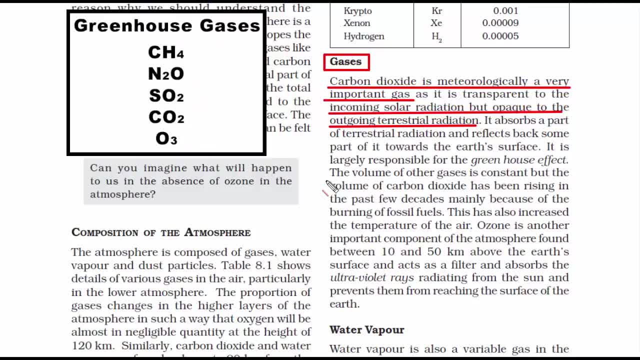 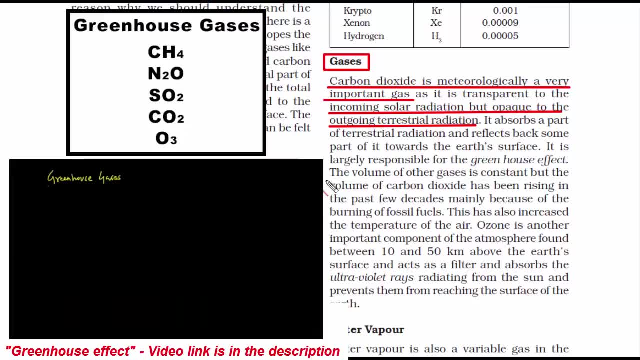 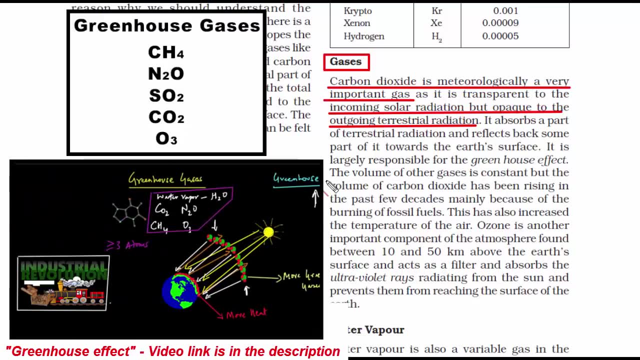 methane, nitrous oxide, sulfur dioxide, ozone, carbon dioxide- So these are bunch of gases in the atmosphere. Now, these greenhouse gases trap the heat within the earth's atmosphere and makes the earth warmer. Now the interesting part to note is that the volume of other gases is constant, but 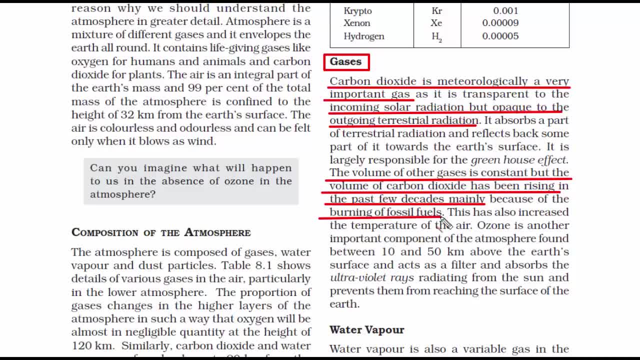 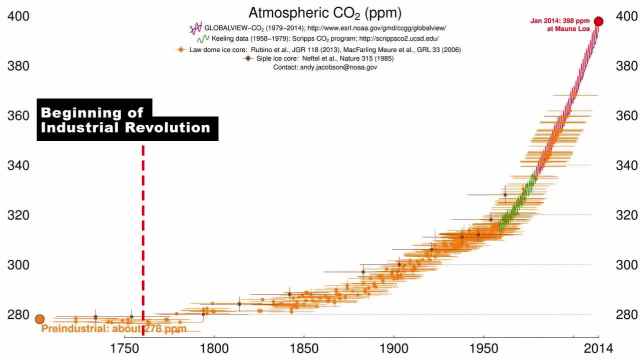 the volume of carbon dioxide has been rising in the past few decades, mainly because of the burning of fossil fuels. Since the industrial revolution, that is, from the mid 18th century, the amount of carbon dioxide has increased. Machines on daily basis are using fossil fuels like diesel, petrol. 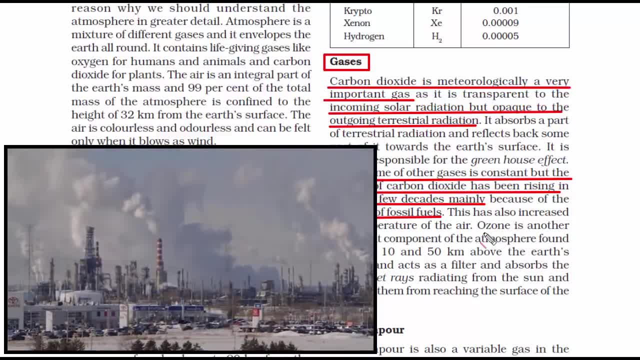 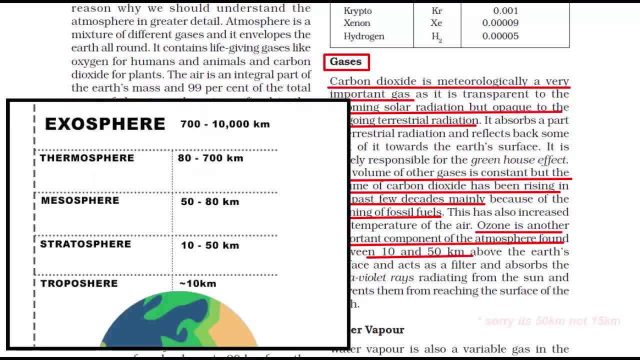 and that's emitting more and more carbon in the atmosphere, which is increasing the overall carbon content. Now, ozone is another important component of the atmosphere that is found between 10 and 15 kilometer above the earth's surface. Basically, it's located in the stratosphere. What ozone layer does? 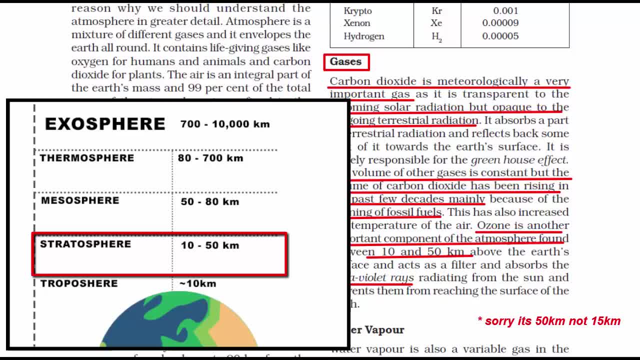 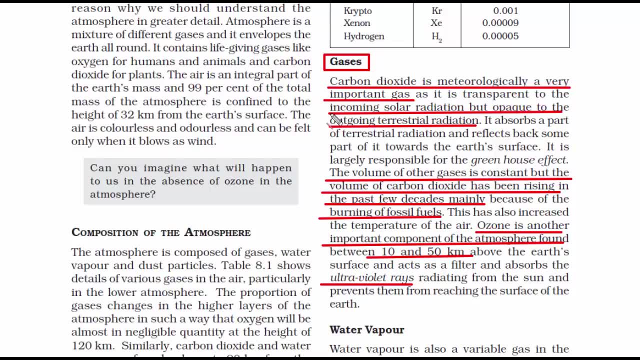 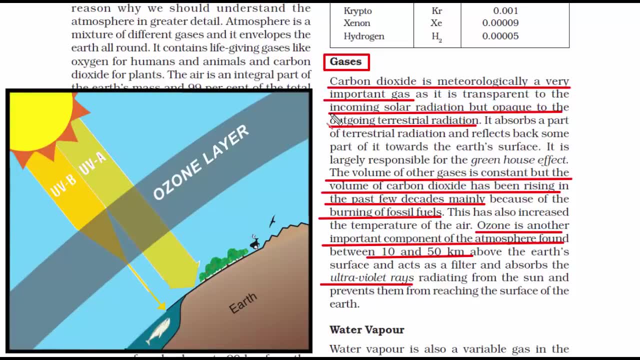 is. it acts as a filter and absorbs the ultraviolet rays that comes from the sun. So UV rays are very harmful. If taken in excess, it can cause sunburn, skin cancer etc. In a nutshell, they are harmful rays. Now, ozone layer is protecting the UV rays from coming directly. Basically, it's filtering it. 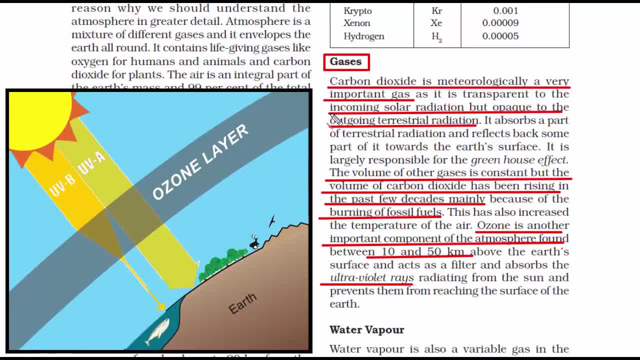 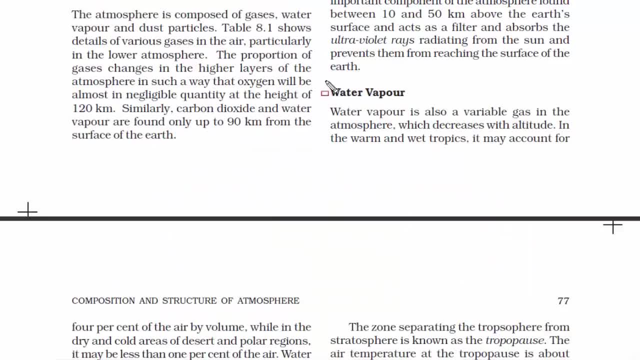 but this layer is depleting. It is purely due to man-made activities. Ozone layer depletion is one of the most serious problems faced by our planet earth. Now we will read about this topic: water vapor. So basically, water vapor is the amount of moisture that is present in the atmosphere. 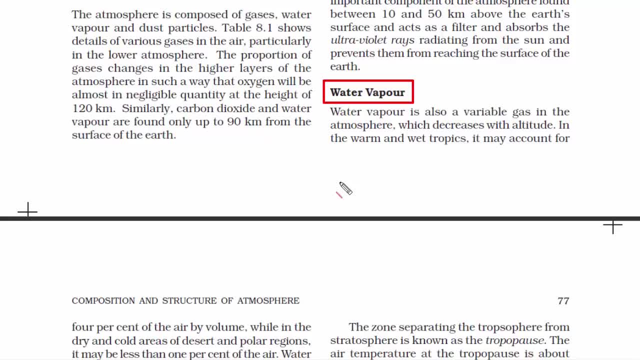 When we think of water, it is in liquid state. With vapor it becomes a gas. So water vapor means liquid gaseous state. So, as I said, the amount of moisture that is present in the atmosphere is called water vapor. Similarly, the amount of water vapor present in the atmosphere is called humidity. And if I were 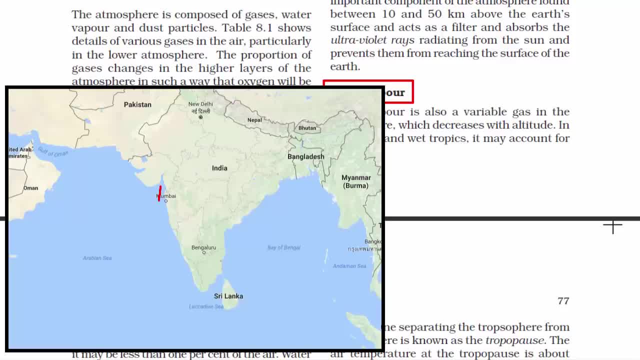 to ask you in India which place is more humid, that would be coastal areas. You go to Goa, Chennai, any coastal place- it's humid because there's a lot of water vapor in the air due to the sea in front of you, And it's not the same case everywhere on earth. The point that I'm trying to make is that 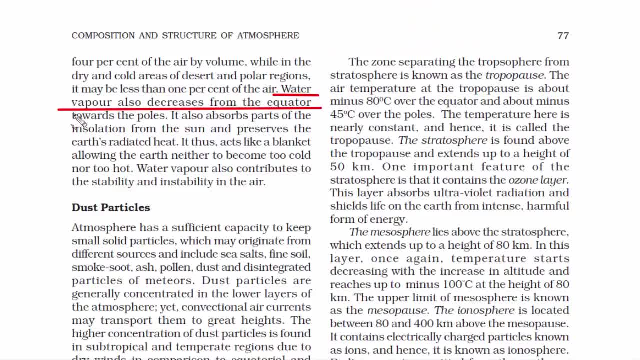 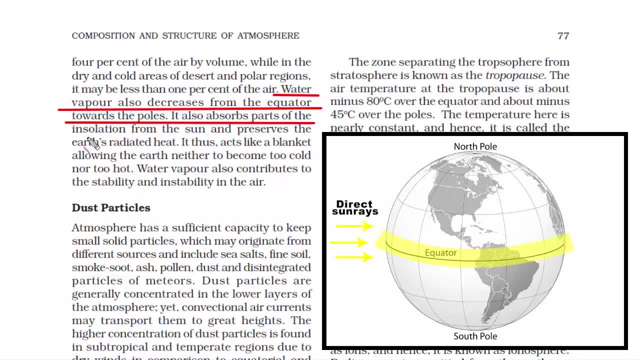 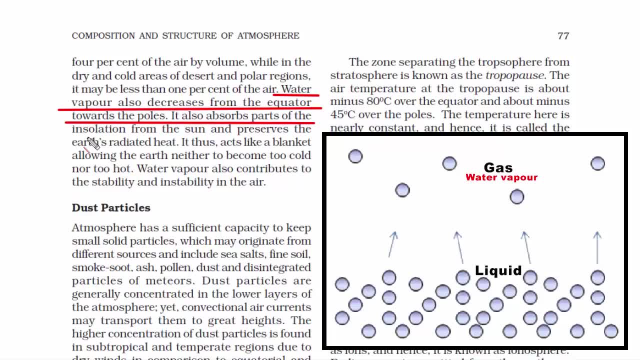 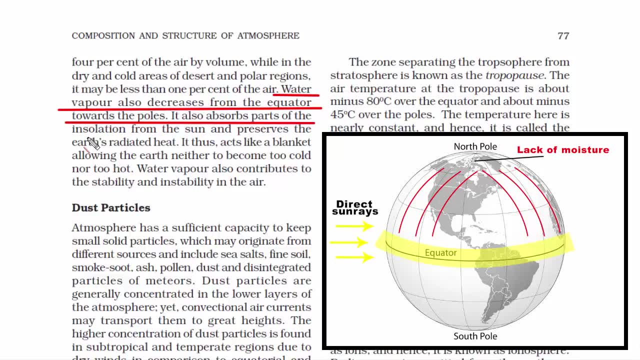 is what increases the water vapor level in the atmosphere. Now, as you go towards the pole area, you will not find moisture. No moisture means no water vapor and no humidity. That's why, when you go to a cold region, your skin will be dry and your lips may crack due to dryness. So this is what is. 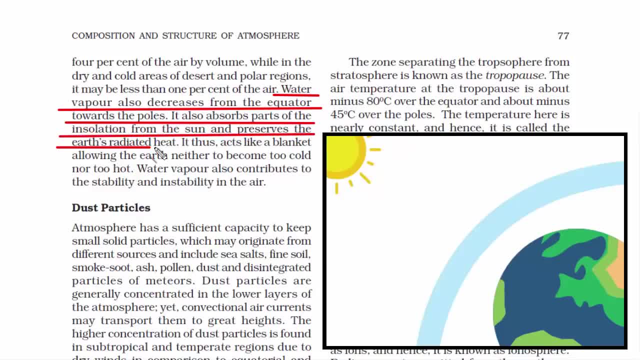 water vapor. Now, the role of water vapor is to absorb parts of the sun rays and not make the earth surface too much warm. Likewise, it also blocks some heat of the sun rays and it does not allow it to escape out of the atmosphere, Because we don't want the entire heat of the earth to escape Without the 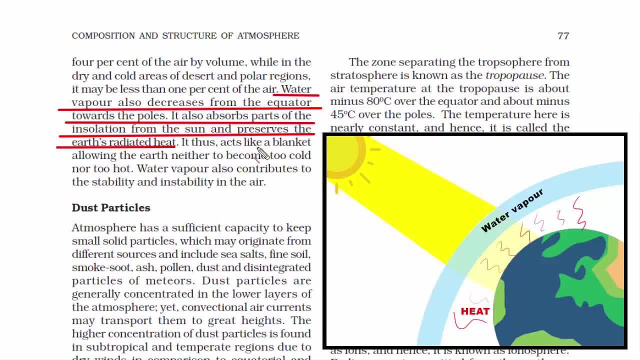 sun's heat, we would have frozen to death. So we need heat, but not too much, and it's the water vapor that sets the right temperature for us to live. It acts like a blanket on the earth, which doesn't make the earth too cold nor too hot. 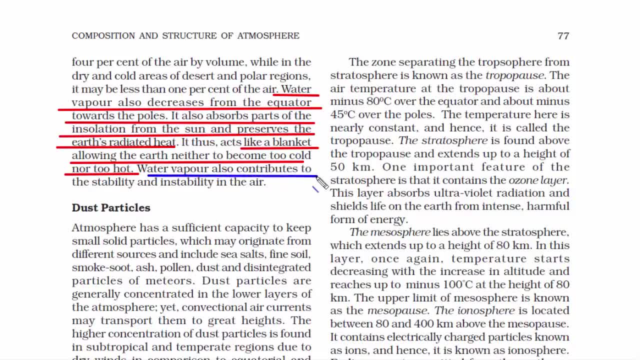 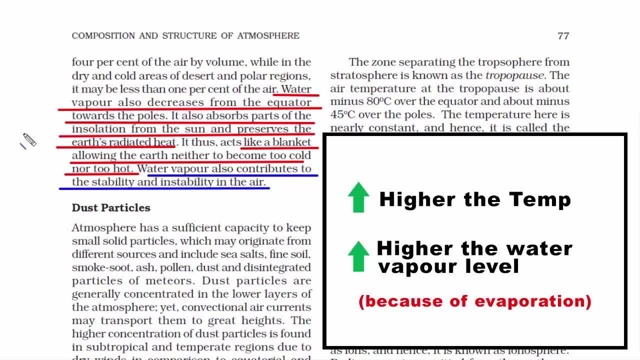 And this line over here is absolutely true- Water vapor also contributes to the stability and instability in the air. Let me just explain this in a simple and straightforward way. The amount of water vapor in the atmosphere exists in direct relation to the temperature. In other words, higher the temperature, higher will be the water vapor content in the atmosphere. 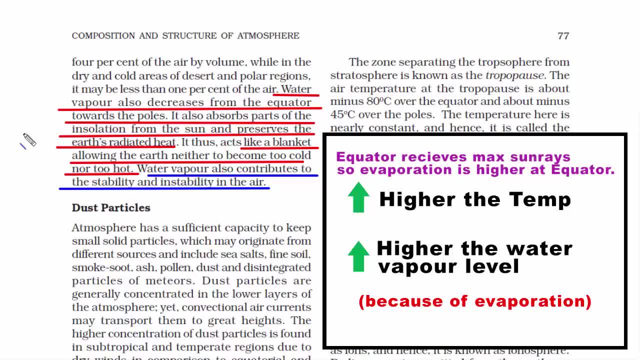 Just like how water vapor decreases as we go away from the equator towards the pole, similarly with increase or decrease in temperature, water vapor also increases and decreases. Now let's assume that I increase the temperature on earth In a more funny or relatable sense. 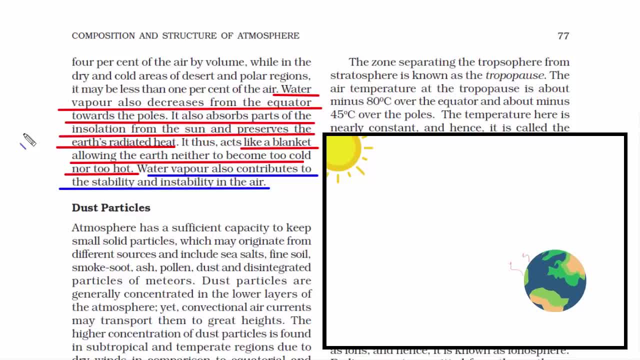 I push the earth a little closer to the sun. That would increase the temperature reasonably. Now more water will evaporate from oceans right, Which means evaporation process creates water vapor. Now imagine this When something else causes an increase in temperature. 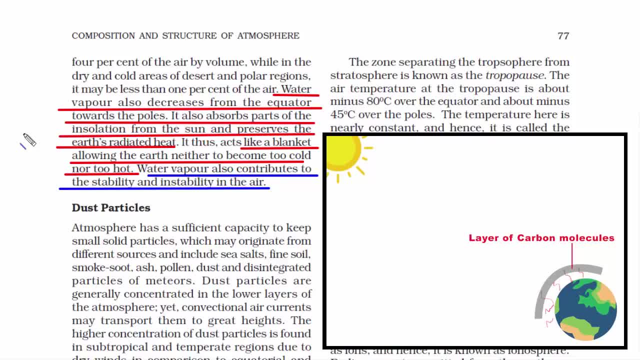 I'm talking about extra carbon dioxide from burning of fossil fuels. so you see here the trigger has changed. Now, instead of me pushing the earth closer to the sun, increase in carbon dioxide in the atmosphere is causing the temperature to rise, Now that the trigger has changed, but the mechanism remains the same. 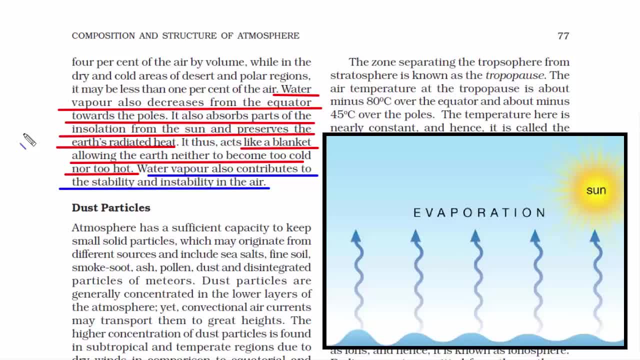 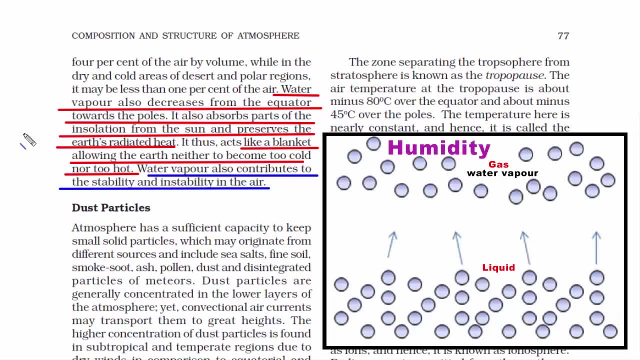 That is due to increase in temperature, more water evaporates. When more water vapor evaporates, more vapor is formed in the atmosphere. An increase in water vapor causes humidity. When there is humidity, we feel warm. Likewise, the air in humid region is warm. 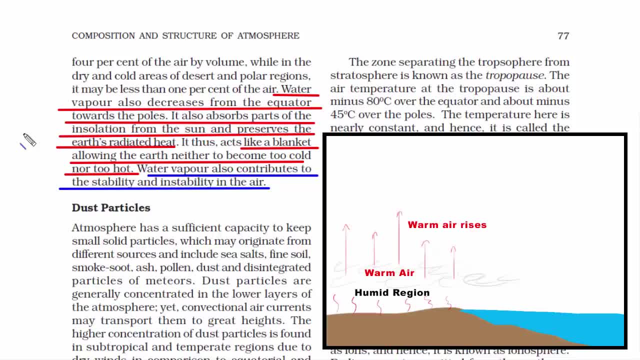 And the warm air rises And that's how it comes in contact with the cool air. When warm air comes in contact with the cool air, turbulence, rainfall and precipitation occurs. So I hope you see the chain effect and you're understanding how water vapor. 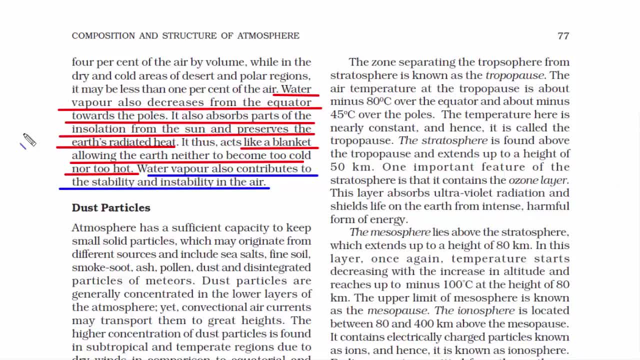 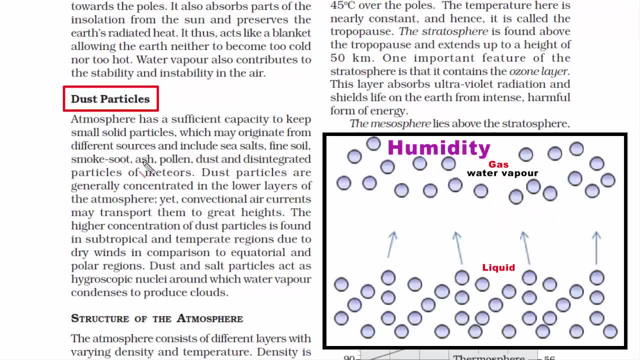 contributes to the stability and instability in the air. I hope you're comprehending as to what I'm saying so far. Now let's talk about dust particles. So far, we saw that there is tons of water vapor in the atmosphere, But I want you to know that. 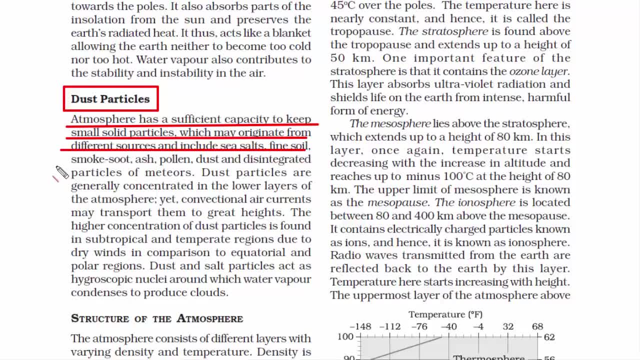 atmosphere has a surface temperature of about 1.5 degrees Celsius. Atmosphere has a surface temperature of about 1.5 degrees Celsius And it has sufficient capacity to keep small solid particles. Now, what are these particles? These are dust particles that originate from sea salts, fine soil, smoke from incomplete burning. 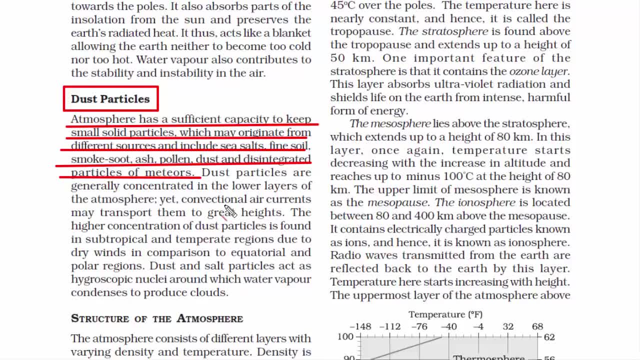 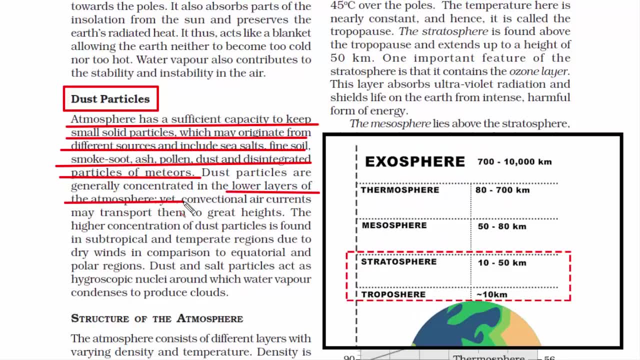 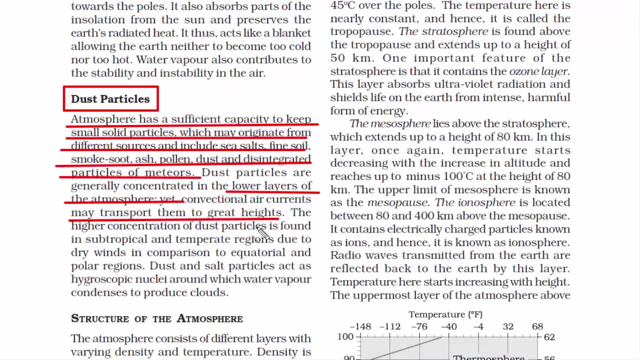 ash pollen, dust and disintegrated particles of meteors. Since dust particles are fairly heavier than water vapor, therefore, they are generally found in the lower layer of the atmosphere, Which are troposphere and stratosphere. Now it is the air movement that takes these dust particles to a greater height. 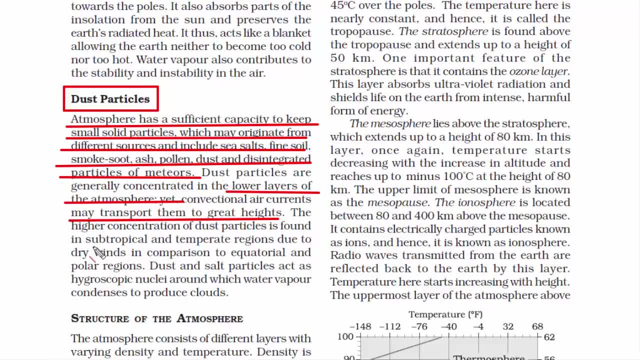 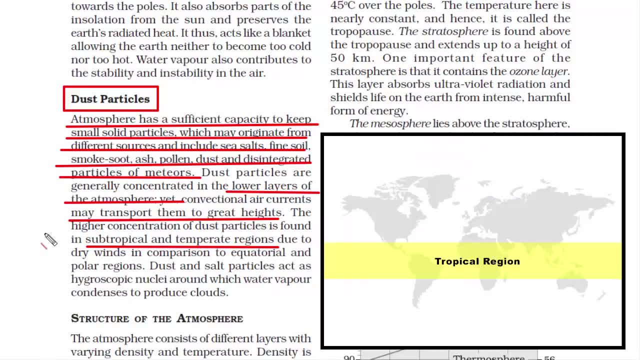 And a longer distance. Now I want you to remember this point: The higher concentration of dust particles is found in subtropical and temperate regions, due to dry winds. I'll show you subtropical and temperate regions on this world map. So here the winds are dry. 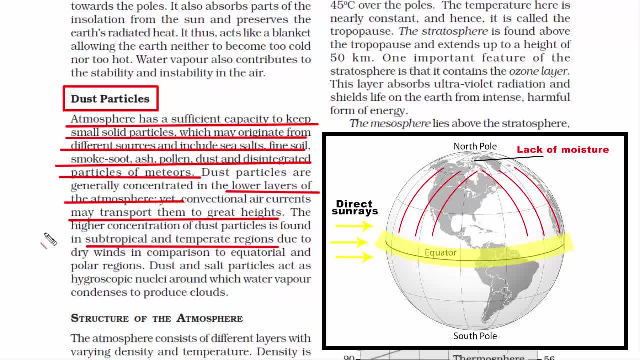 Remember moments back we read that water vapor decreases as we go away from the equator towards the poles. That means at equatorial region the moisture content in the atmosphere does not allow the dust particles to rise. But then, as we go away from the equatorial region, 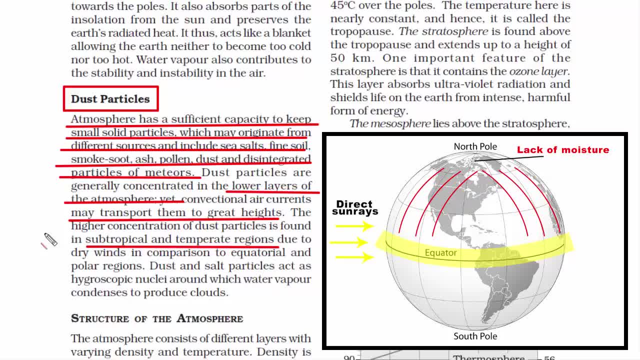 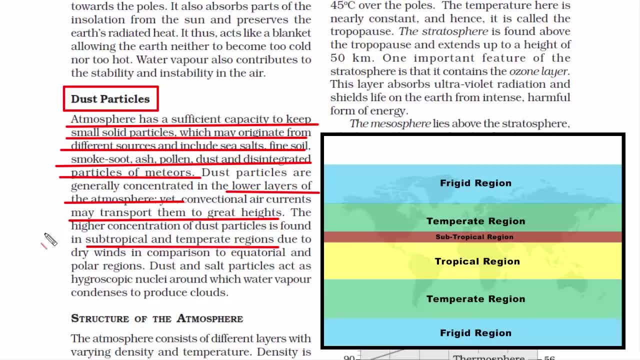 away from the equatorial region, moisture content in the atmosphere decreases and dry wind carries the dust particles. and as we go further away at poles area- I'm talking about North Pole and South Pole- there you will hardly find any dust particle. you will mostly see ice crystals. I don't know if that can be. 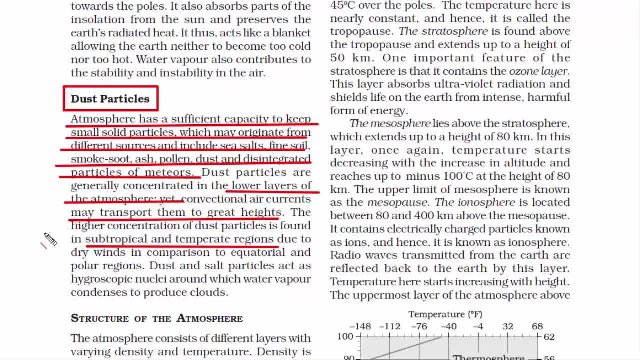 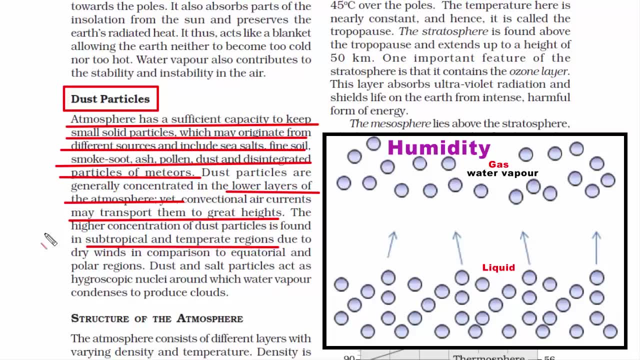 called as dust particle. another important point is that dust particles are a major component behind cloud formation. now, if you see, there is water around us all the time in the form of tiny gas particles, which is also known as water vapor, then there are also tiny dust particles floating around in the 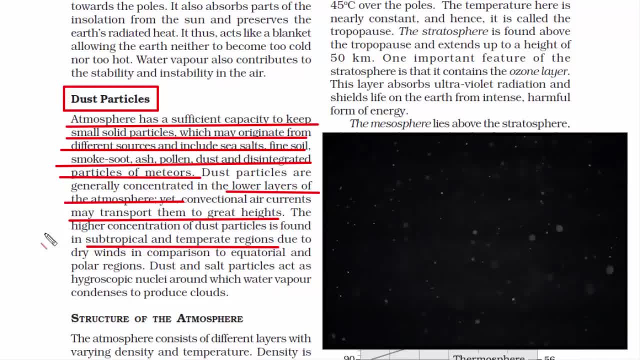 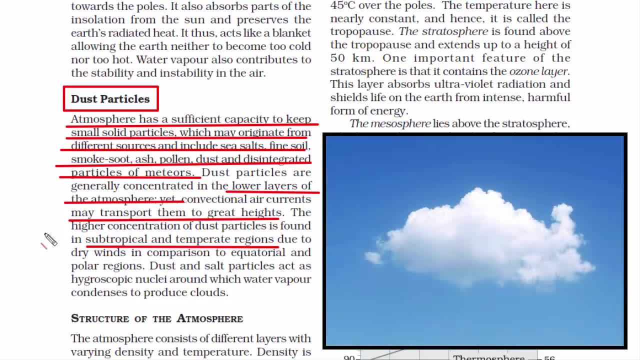 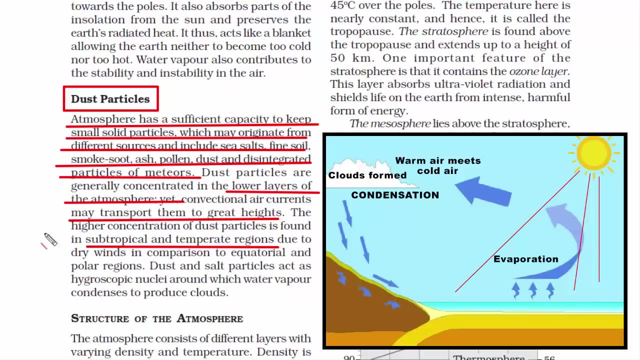 air. now if you look closely at a black background, you can see the dust particles. so the combination of this water vapor and dust particles together forms a cloud. obviously you must have heard that cloud is a result of condensation, where the water vapor turns into visible water droplets. but then if 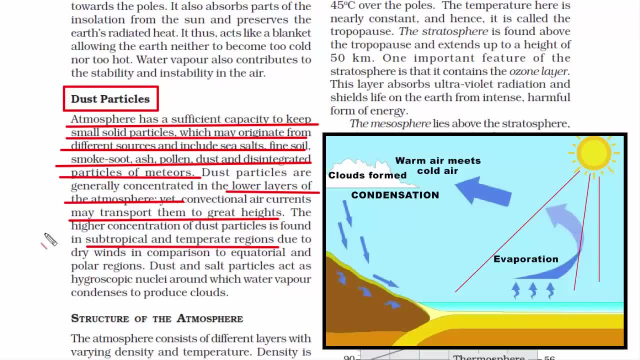 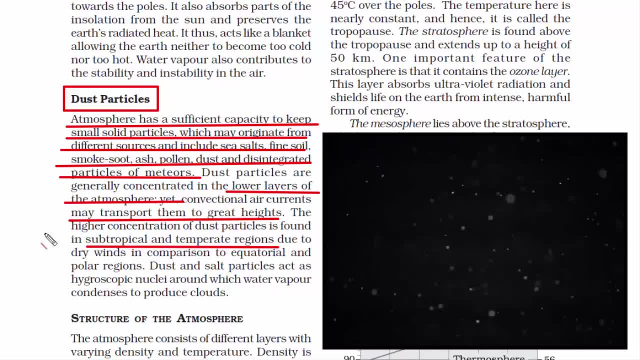 there isn't anything to hold them up in the air, how will a cloud form? otherwise droplets will fall and it will simply rain. so to hold this kind of particles in the air we need to have a seeing kind of a cloud. this condensed water droplet, floating dust particles come into picture. These 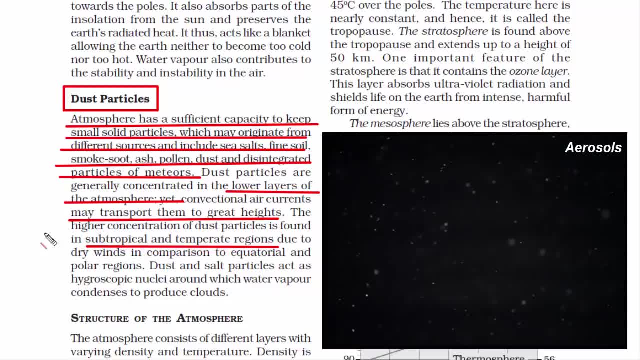 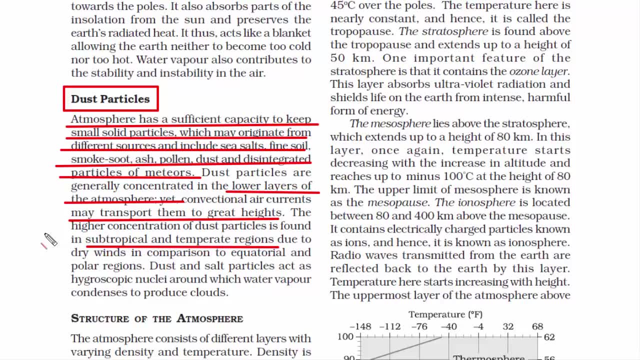 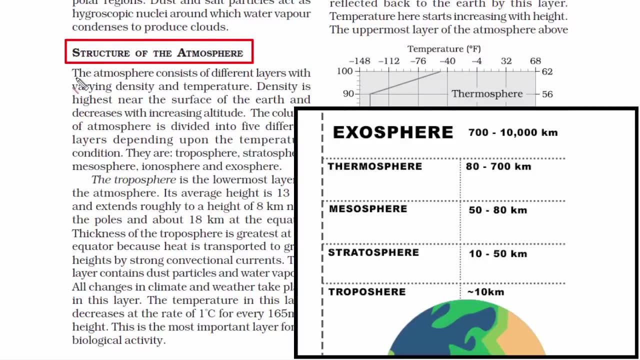 are called aerosols. These aerosols attract the condensed water droplets and large combination of these forms a cloud. So that's the role of dust particles. Now let's get to know quickly about different layers of the atmosphere. So this is a picture of different layers of the atmosphere, From low most layer, to 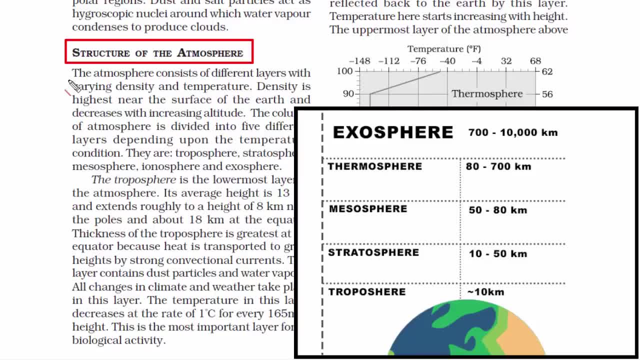 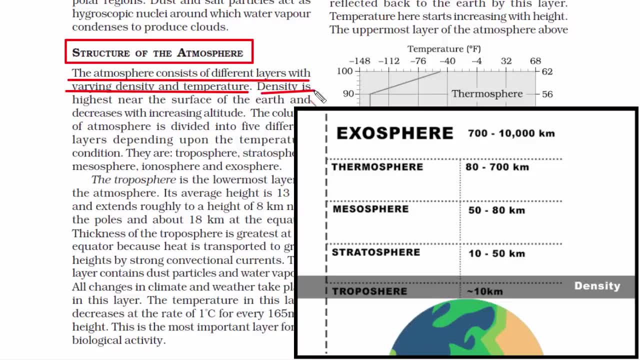 the outer most layer. overall, there are five layers. Remember this order. Now these layers have different density and temperature. Now density is highest near the surface of the earth because of the gravitational pull of the earth, And as we go higher, the density decreases. Now, coming to the temperature part, the 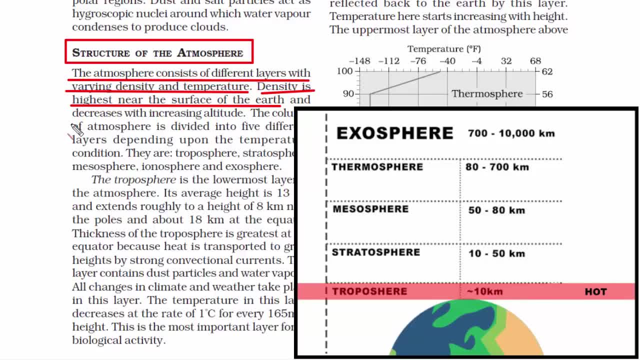 lowest layer, that is, the troposphere, is hotter because it's nearer to the earth surface. So heat from the earth warms up the air of this layer. As the height increases, the number of air molecules decreases, and that's how temperature decreases, And this continues till the end of 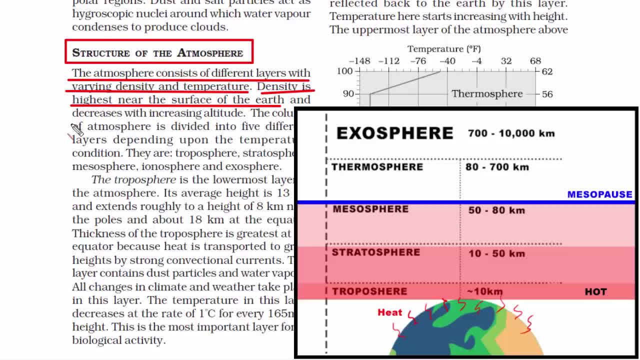 Mere Now. this place is also called as mesopause. This is the coldest part of Earth's atmosphere. Temperature falls up to minus 90 degrees Celsius. Now, after mesosphere, we have thermosphere. By the word thermo you can relate the word. 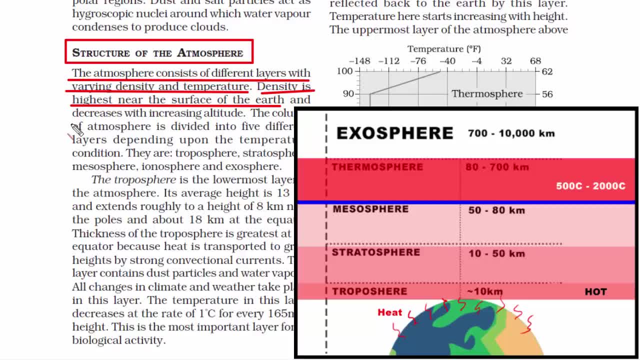 thermal, and which means heat. Here the temperature goes up to 500 to 2000 degrees Celsius. Now, after this, we have exosphere. It is also the first layer to come into contact and protect the earth from meteors, asteroids, comets and 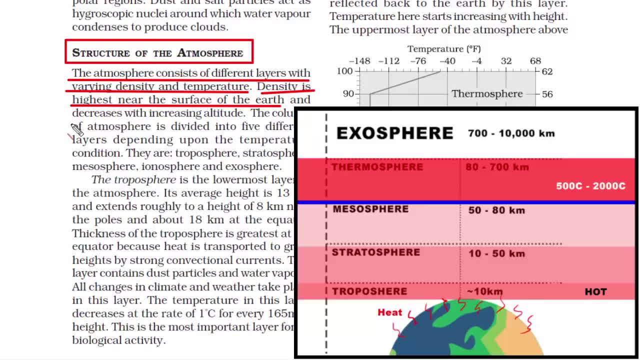 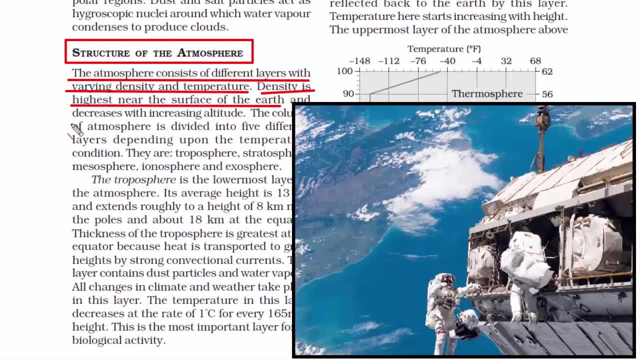 comets Basically after this layer, space starts. The temperature here varies from zero to over 1700 degrees Celsius. That means it is colder at night and much hotter during day. And I also remember watching some NASA astronauts interview where he said that when an astronaut goes on a spacewalk, that space suit they 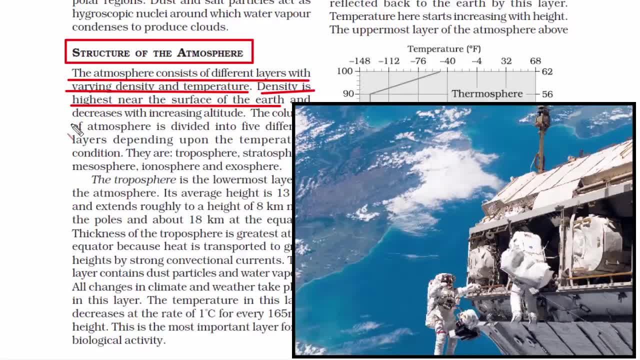 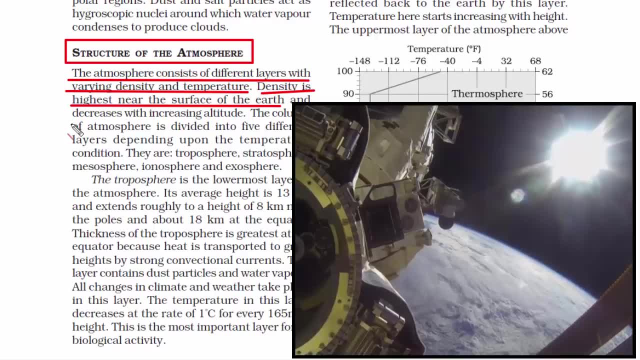 are wearing. it is like the mini spaceship. It protects them from the heat of Sun. and he said something which I will always remember. He said: when they face the side where the Sun is, that side is illuminated by the Sun. As a result, that front part of 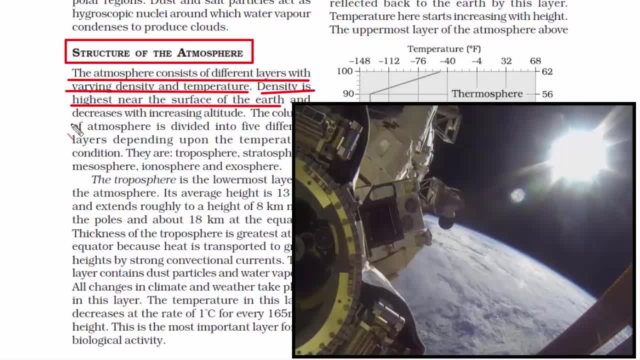 the suit is so much hot and the back side of the suit is freezing cold. I hope you are getting what I am saying. Of course, the space suit has the temperature control mechanism, which keeps the astronauts safe, But I hope you are getting the relevance of the extreme sides of the atmosphere.